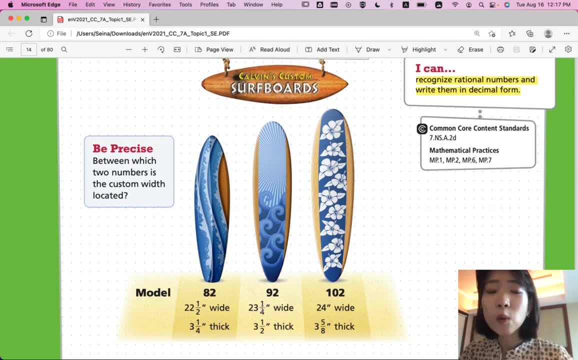 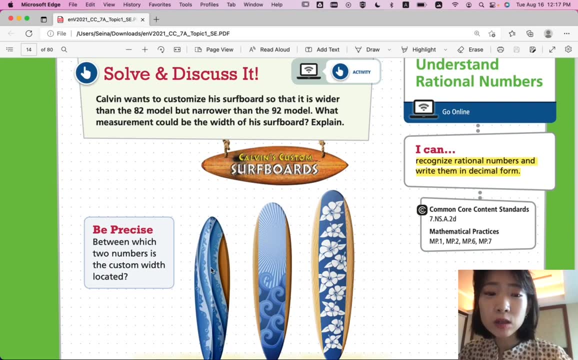 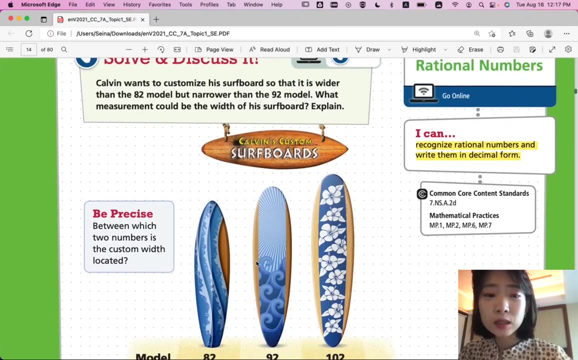 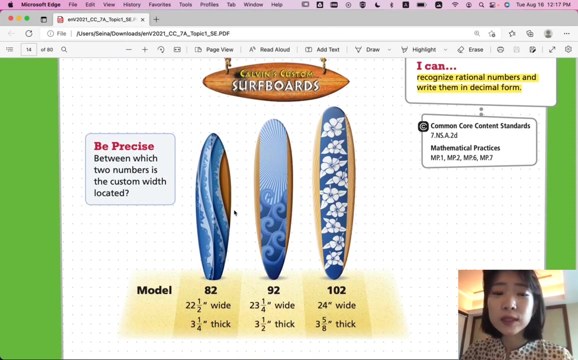 And model 92.. 22 is 23 and 1 fourth inches wide. So if it's wider than 82 model, but narrower, so like smaller than the 92 model, what measurement could be the width of his surfboard? So he has a separate surfboard, okay, So if it's wider than this one but narrower than this one, what number could come between 22 and 1 fourth, 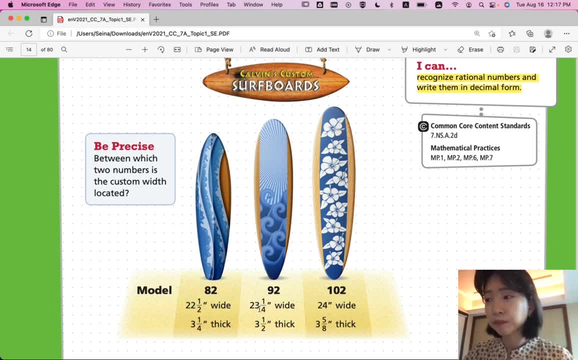 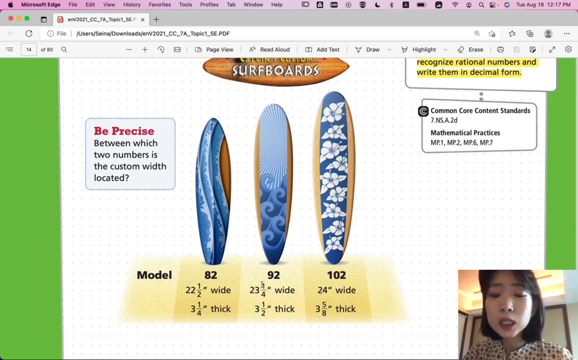 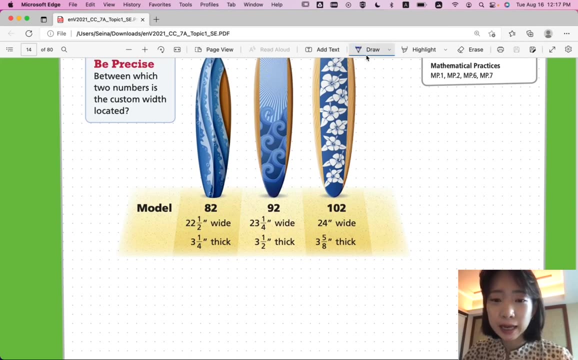 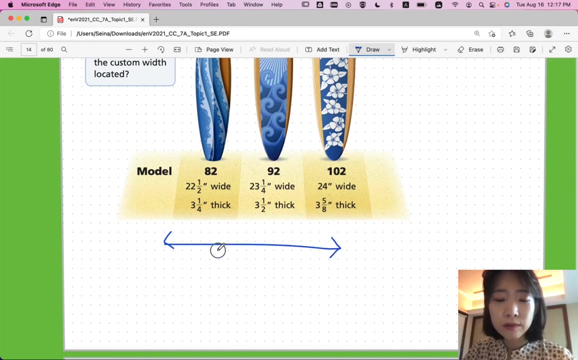 two and a half and 23 and 1: 4th. it should be between these two, right? so a nice little whole number that's between these. is it 22, 23 or 24? in order to better understand, you can draw a number line. so if that is 22 and you have 23, 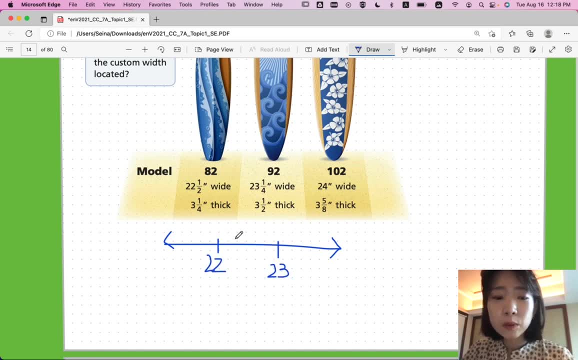 here 22- point half is right here, okay. and 23 and 1: 4th. if that is 24, this is half and that's 1: 4th. so that is right here. so if his another surfboard is between these two and you want a whole number, you can say it's. 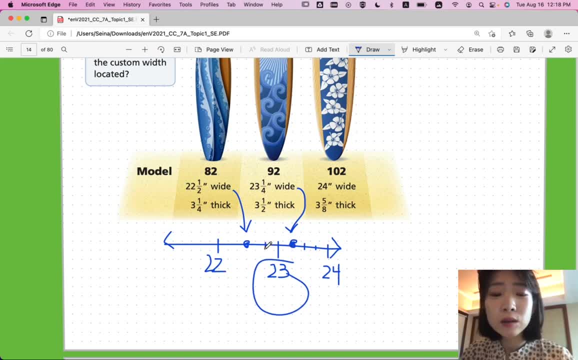 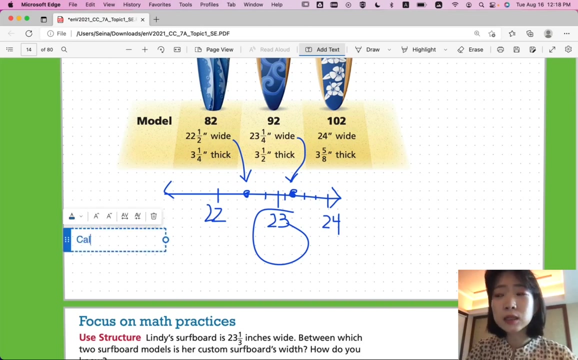 20- 23, or you can do 22 and 3- 4th, or 23 and 1- 8th. okay, there could be numerous possible answers, but if you want a whole number, you can say it's 23 inches. it could be 23 inches, so let's write that down. Calvin's surfboard should be. 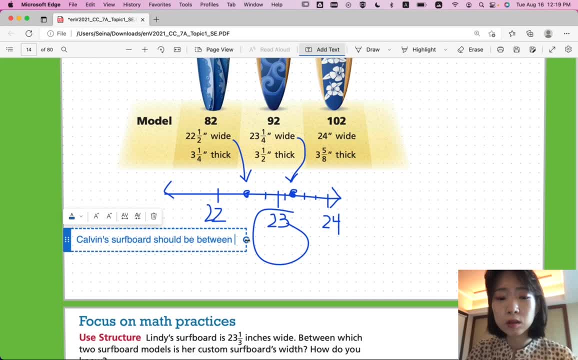 between 22 and 1 half inches and 23 and 1, 4 inches wide. the width of his surfboard could be 23 inches. okay, so let's look at focus points to get the full definition of focus points. okay, so let's look at focus points to get the full definition of focus points. 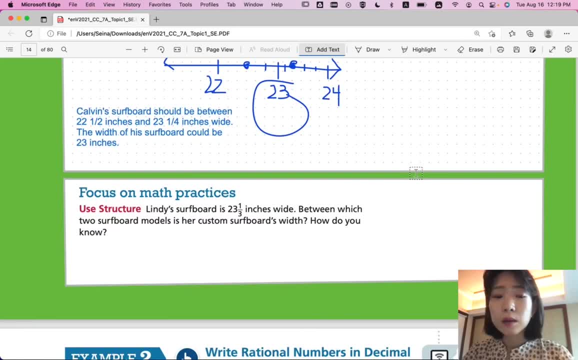 So let's look at Focus on Math Practices. Linda's surfboard is 23 and 1 third inches wide. Between which two surfboard models is her custom surfboard's width? How do you know? So, if Linda's surfboard is 23 and 1 third inches wide, look at the widths here. 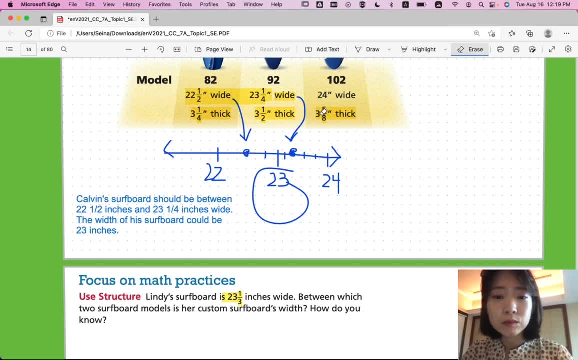 Where does it lie between? So 23 and 1 third is greater than 23.. Is it greater than 1 fourth or is it less than 1 fourth? If its less than 1 fourth, it's between models 82 and 92.. 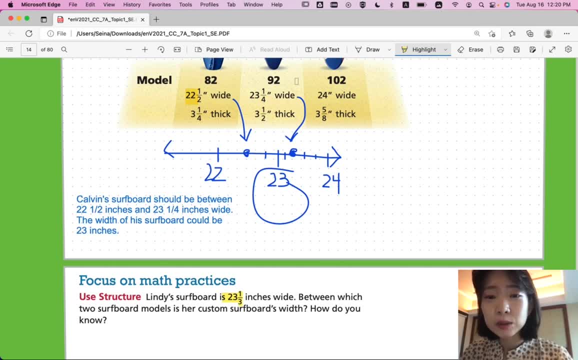 If 23 and 1 third is greater than 1 third, it's between models 82 and 92. Where does it lie between one-fourth? it's between it's probably between 92 and 102. so look at the number line again: 23 and one-third is around here, so it's really close to one-fourth. 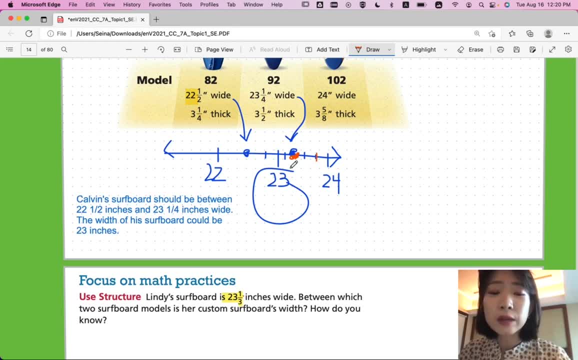 but it's one-fourth smaller or greater than one-third, is the question. if you change this to decimal, one divided by three is zero. point three, three, three repeated right. and what about one-fourth? one-fourth one divided by four is 0.25. 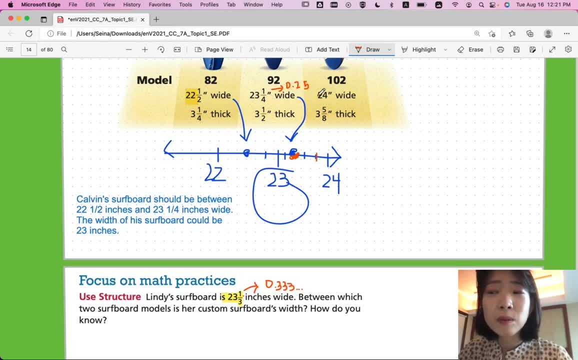 exactly 0.25. is 0.25 smaller or or greater than 0.333? dot dot, dot. yes. two on the tenth place is smaller than three. so lindy surfboard is wider than model 92, so it's going to be between 92 and 102, model 92 and 102, and 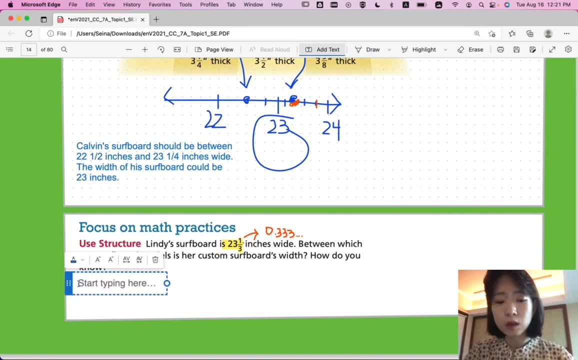 and let's explain how we know. so, between the 92 and 102 models will be our answer. 23 and 1. 3rd is greater than 23 and 1 4th and less than 24, because one third is greater than one fourth, one third. 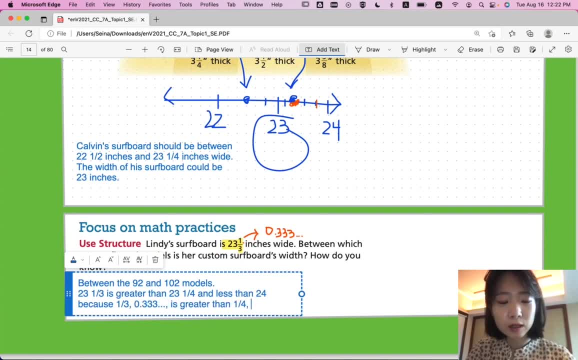 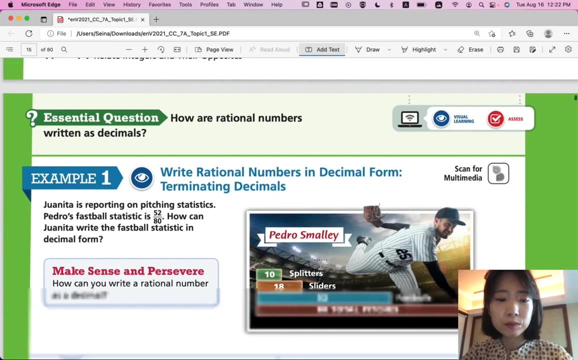 three, three, three repeated is greater than one fourth, 0.25. okay, so you can draw a number line to compare them and if they're too close you can change them into decimals to compare them to. okay, let's look at the next page. so throughout this lesson, let's think about how are rational numbers written as: 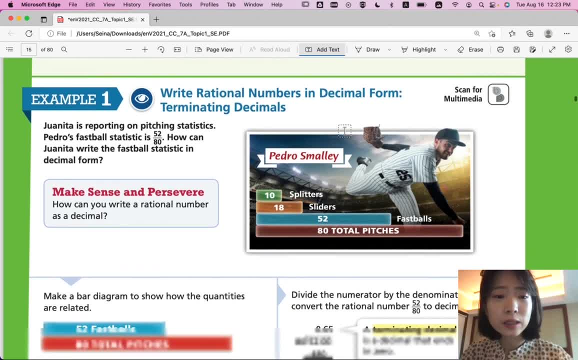 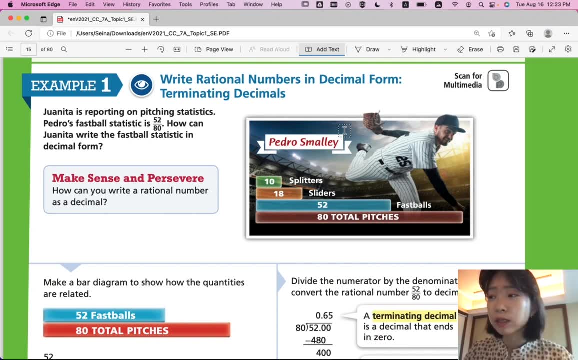 decimals. example one: write rational numbers in decimal form. terminating decimals. so decimal has different um types. okay, terminating decimals. do you know what terminating means? to terminate, terminate, terminate, terminate, terminate, terminate, terminate. you might think of repeating decimals, but terminating is not repeating. terminating means to end, so it means decimals. that has an ending. okay. 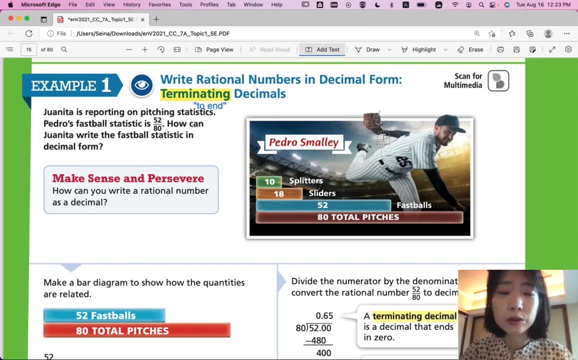 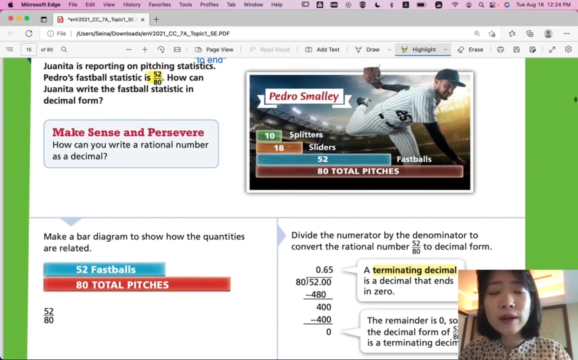 so decimals. that has an exact solution. that ends at some point. Juanita is reporting on pitching statistics. Pedro's fastball statistics is 52 over 80. how can Juanita write the fastball statistic in decimal form? so how can we write 52 over 80 in decimal form? you will, in order to write fraction. 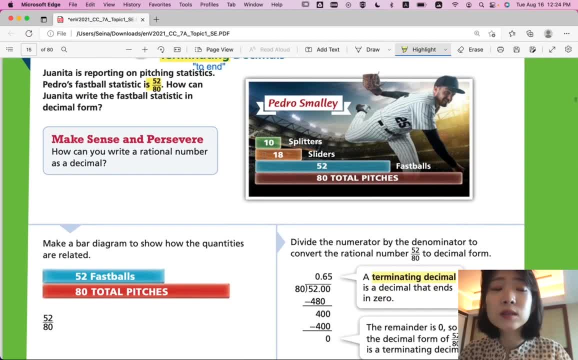 to decimal. it's fairly easy, you will. you will literally divide the numerator by the denominator. because what does the fraction bars represent? it means division. 52 divided by 80 is literally 52 divided by 80. okay, 52 divided by 80. so you're literally gonna divide 52 by 80. so you will get, you will eventually. 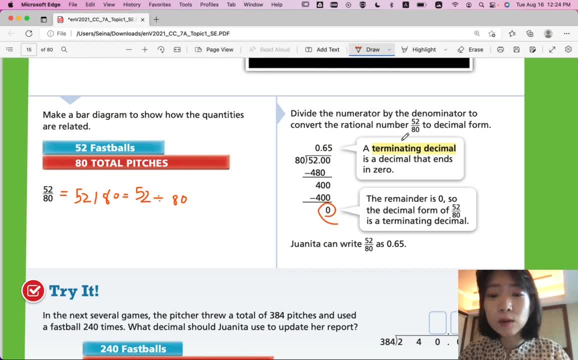 get 0.65 with a remainder of 0, which means this is a terminating decimal. okay, a terminating decimal. write this in your graphic organizer in the beginning of the topic: terminating decimal is a decimal that ends in 0, so Juanita can write 52 over 80. 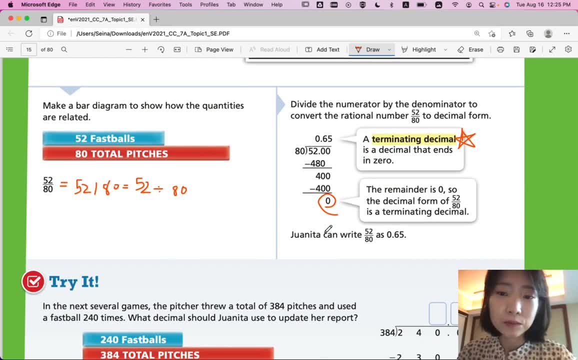 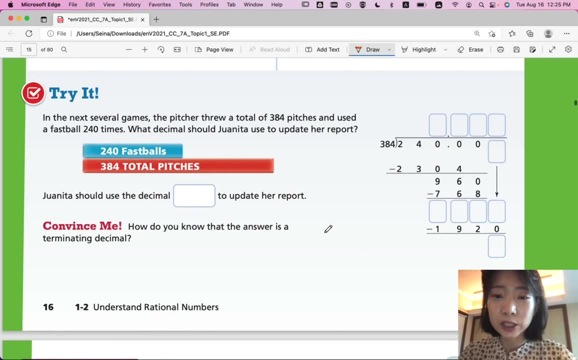 0.65. let's look at triad question. in the next several games the pitcher threw a total of 384 pitches and used the fastball 240 times. what decimal should Juanita use to update her report? see if you can fill in the blanks by yourself. 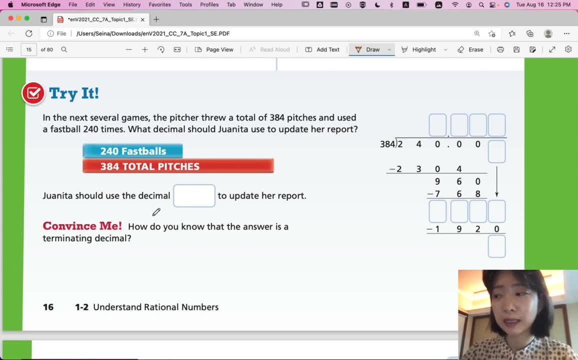 and figure out the answer by yourself. come back when you're ready for answer. okay, are you ready? so divide 240 by 384. 384 doesn't go into 240, it's greater than 240, right? so you're gonna start with 0 here and then pull down the 0 and see how many 384s. 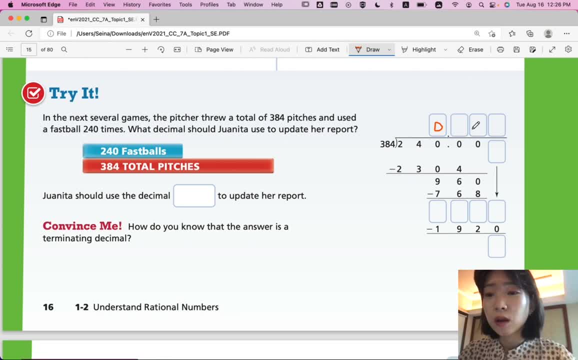 going to you 2,400 now and you will get 444 forward. 184. now here you got to try. 6 times 384 is 2304.. Find the difference, bring down the 0, and see how many 384 goes into 960.. 2 times 384 is 768.. And the difference 192,. bring down another 0. 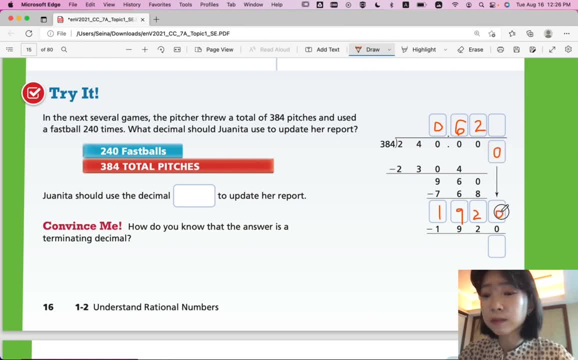 by annexing a 0 here And 384 times 5 is exactly 1902.. So you get a remainder of 0.. So Juanita should use decimal 0.625 to update her report. Convince me. how do you know that? 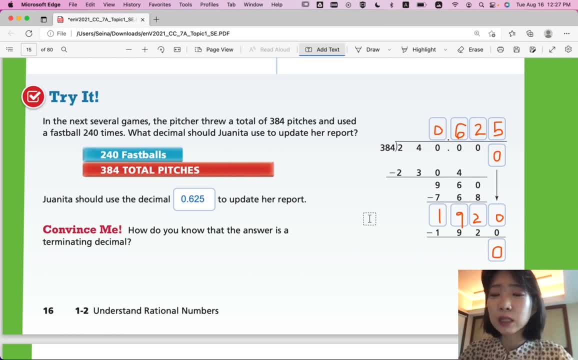 the answer is a terminating decimal. How do you know if it's terminating or repeating? How do you know if it's terminating or repeating? How do you know if it's going to keep going or not? Because when you have a remainder of 0, then you're done dividing right. It's just going to be 0, 0, 0. So you're going. 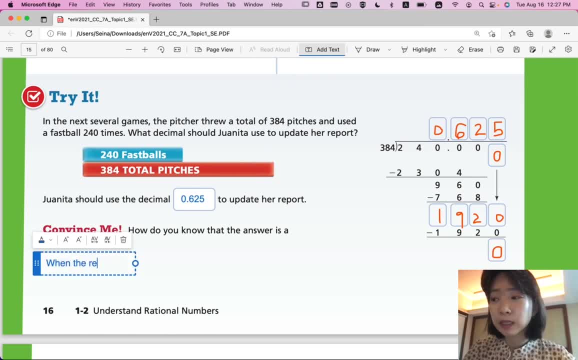 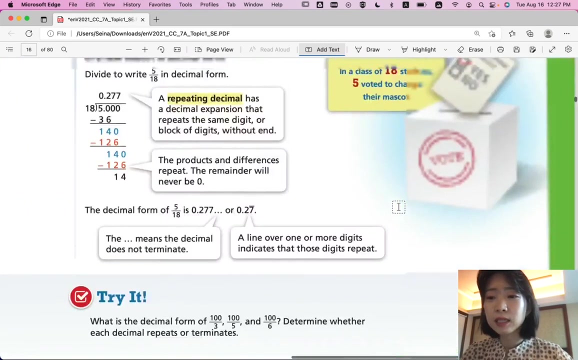 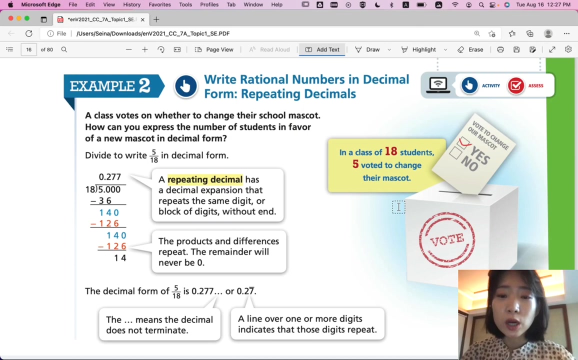 to end with 0. So when the remainder is 0, the decimal is a terminating decimal, because there are no parts left to divide. And you're done. Okay, Let's look at the next page, Example 2.. Write rational numbers in decimal form: Repeating decimals. So now we're going to. 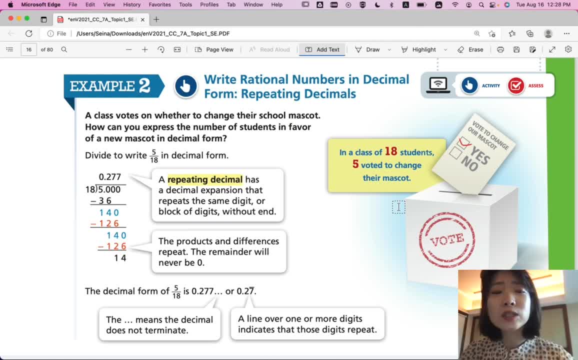 look at repeating decimals. A class votes on whether to change the number of numbers to change their school mascot. How can you express the number of students in favor of a new mascot in decimal form? So in a class of 18 students, 5 voted to change their mascot. 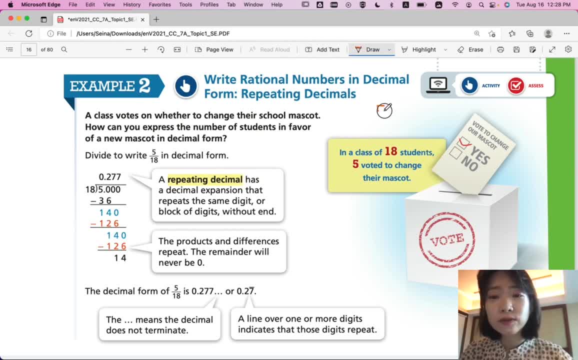 So we're going to have a fraction of 5 out of the whole 18 students. Okay, So write this in a decimal form: When we divide 5 by 18, we have 0.277.. And then we'll notice that we get the exact same remainder every time: 14 and 14.. And 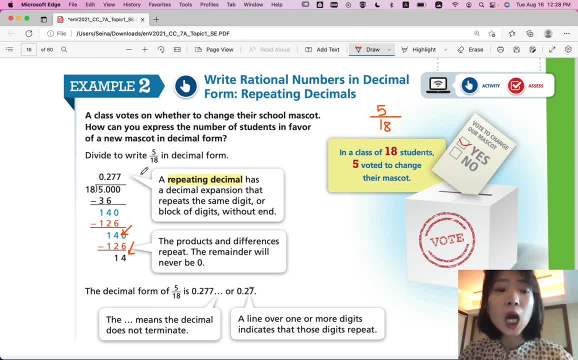 you're going to keep getting 14 as a remainder And you're keep going to say 7.. You're keep going to multiply 18 by 7, right, So that's a repeating decimal. Write this in your vocab graphic, organizer. Repeating decimal has a decimal expansion that repeats the same digit. 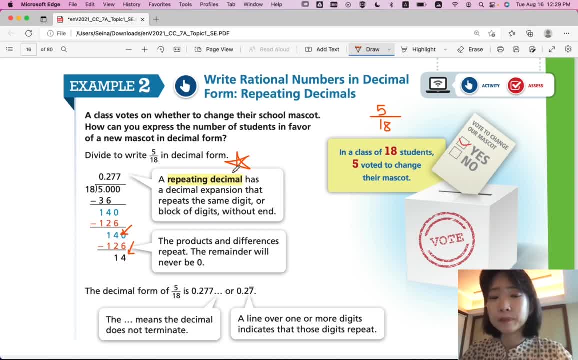 or block of digits. So it's keep going to repeat 777.. The products and differences repeat. The remainder will never be 0. It's never going to end. It's keep going to repeat itself. So the decimal form of 5 or 18 is 0.277.. or you can write a repeating bar over the digit that is repeating. 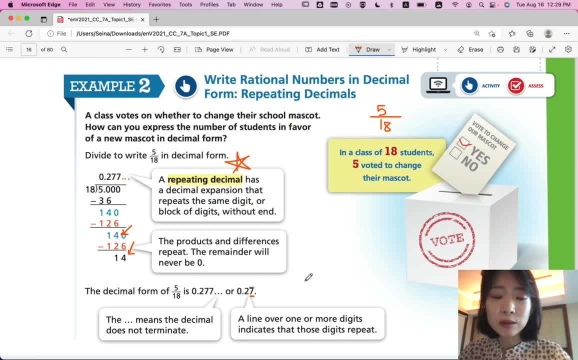 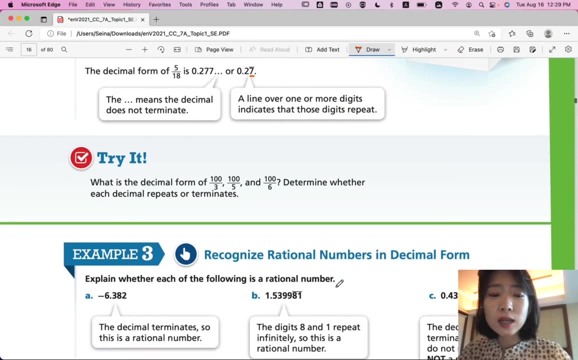 So if you have 2 digits or 3 digits or more digits that are repeating, put a repeating bar over all the repeating decimals. Okay, So let's look at triad. What is the decimal form of 100 over 3,, 100 over 5, and 100 over? 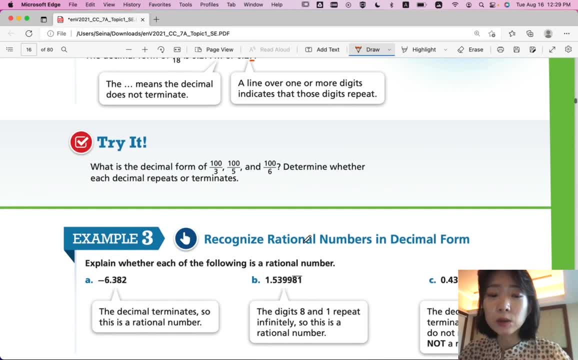 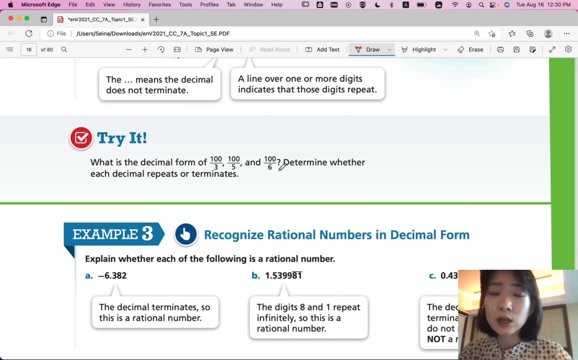 6? Determine whether each decimal repeats or terminates. So divide 100 by 3, 100 by and hundred by six and determine if any of them are repeating decimal or terminating decimal. okay, pause the video and solve it by yourself. come back when you're ready for answer. okay, are you ready? 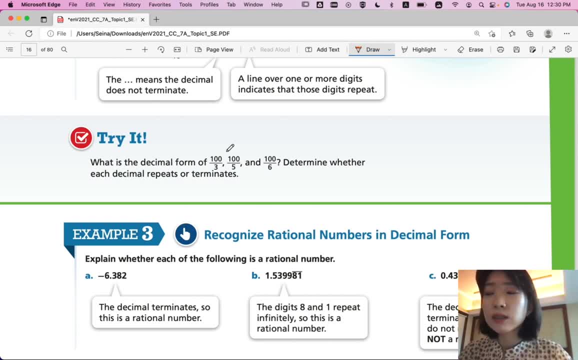 so, a hundred divided by three, you should get thirty three point three, three, three repeated, or you'll write 30.3. repeat it here, okay, and hundred over five. you will get hundred, Oh, divided by six, and determine if any of them are repeating decimal. okay, stop, pause the video and solve it by yourself. come back when you're ready. pause the video and solve it by yourself. come back and. 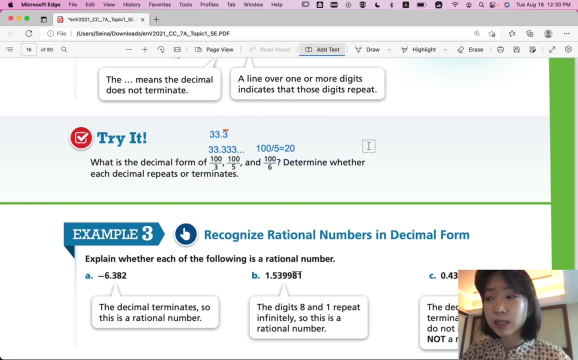 by 5 is exactly 20.. So that is a terminating decimal, or rather a whole number. And 100 divided by 6 is 16.6666 repeated, So you will have 16.6 bar here. Okay, So this one is repeating. 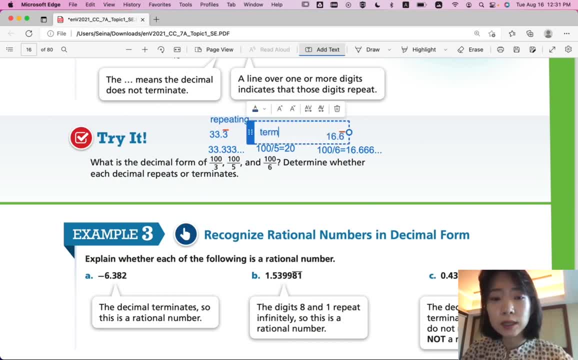 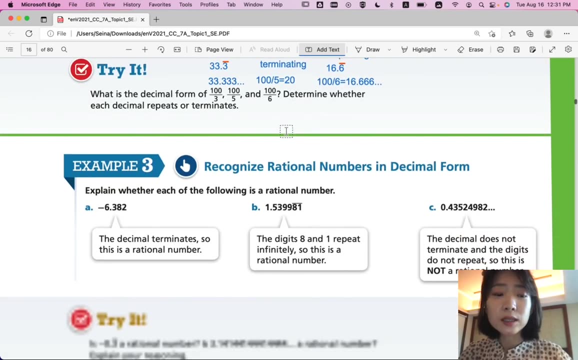 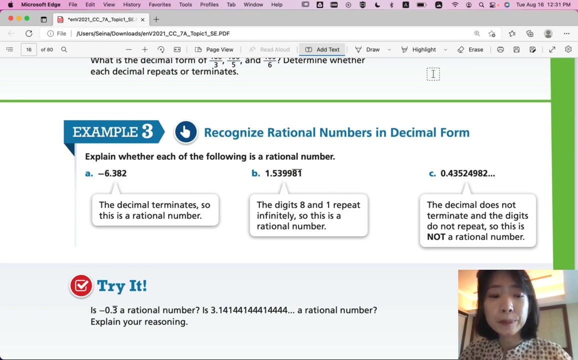 and this one is terminating and this one is repeating. Okay, let's look at example 3.. Recognize rational numbers in decimal form. Explain whether each of the following is a rational number: Negative: 6.382.. This decimal terminates. It doesn't have a dot dot dot or a bar that says it's repeating. So this is a. 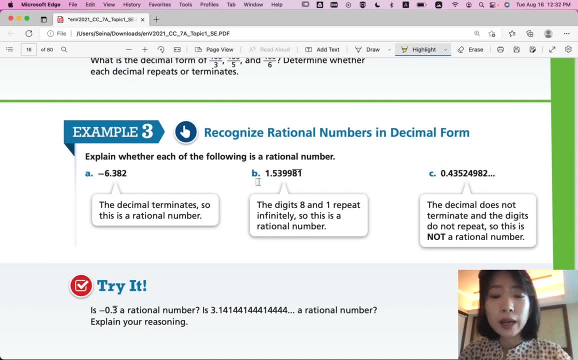 rational number, Okay, the digits. Let's look at part B: 1.539981.. 8- 1 repeats right. The digits 8 and 1 repeat infinitely, But this could also be written as a fraction. So it's a rational number, Okay. And part C. 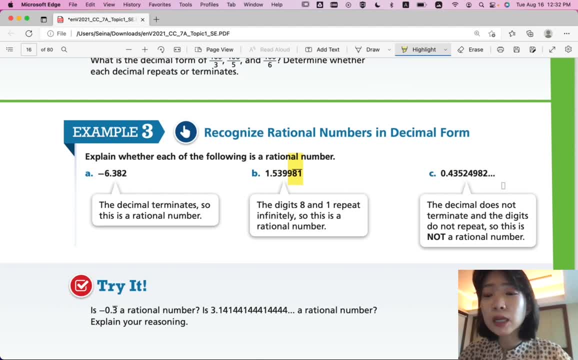 0.43524982.. Does it have a pattern? It is not repeating or it is not terminating. So if it's neither of those 2 types of decimals, it is not a rational number. Yes, it is a decimal, but it doesn't go into the category of repeating. 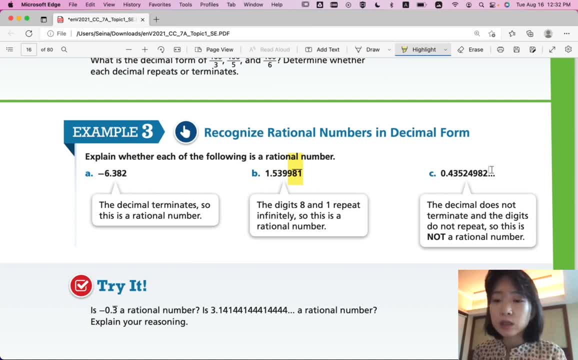 decimal or terminating decimal. So in this case this is NOT a rational number. Next rational number: okay. so if it terminates or if it repeats, it is a rational number. if it doesn't do any of those, it is not a rational number. okay, look at the triad. 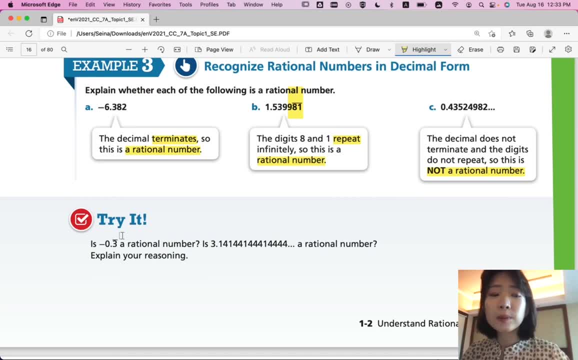 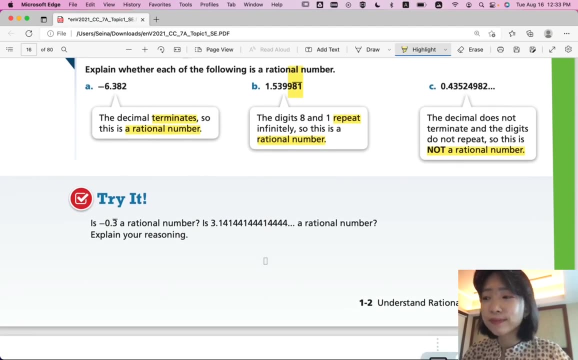 is negative zero. point three: repeated. a rational number is three. point one: four, one four, four. one four, four, four one four, four, four, four, dot dot dot. a rational number. explain your reasoning. okay, is the first one a rational number? it is a repeating decimal. so, yes, that decimal value repeats, so negative zero. 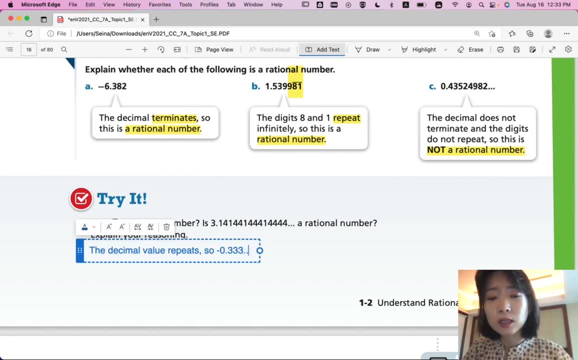 point three, three, three, dot, dot dot is a rational number. all right, let's do. let's do this. okay, what about three point one four, one, four, four, one, four, four, four, one, four, four, four, four, dot, dot dot. it does have a pattern, but is it repeating, it seems. 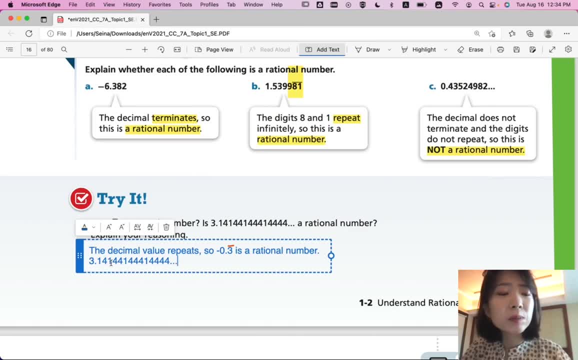 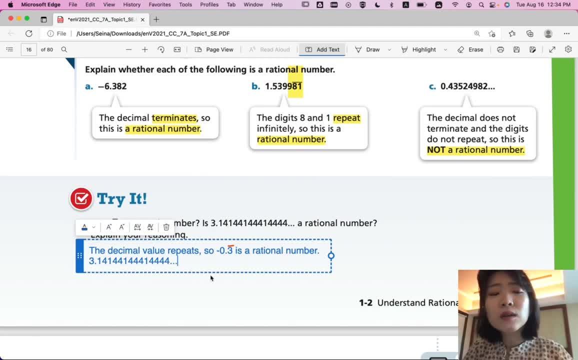 different number of digits. right, so it does have a pattern, but it's not a repeating decimal, okay. it does not terminate or repeat, so it is not a rational number. okay, so be careful with these type of decimals. it does look like it's repeating something, but just because it has a pattern. 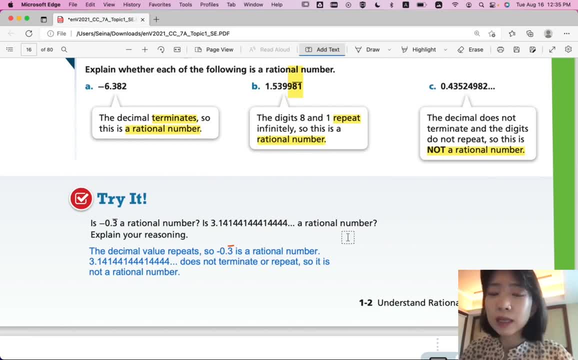 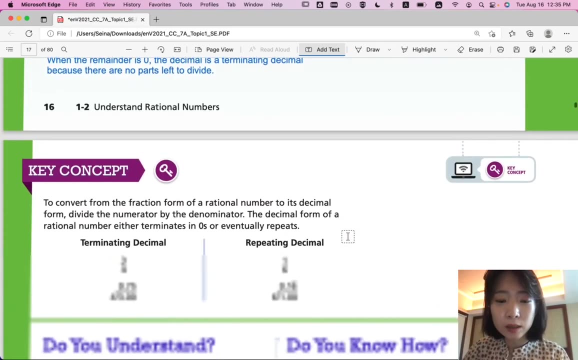 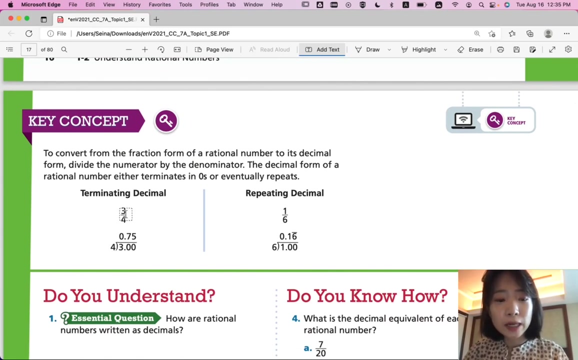 doesn't mean it's a repeating decimal. okay. it needs to have an exact amount of the same digits that are repeating. if not, it is not a repeating decimal, okay. keeping that in mind, let's wrap up our lesson. so, to convert from the fraction form of a rational number to its decimal form, you're gonna divide the numerator. 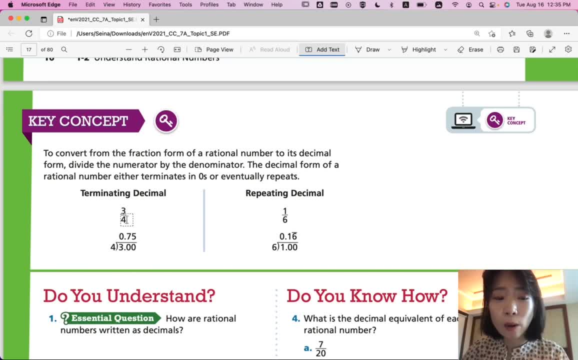 by the denominator. you literally divide three by four and one by six to get the decimal form. the decimal form of a rational number either should terminate in zeros or eventually repeats. if it's neither of those decimal, it is not. it cannot come from fraction, it cannot be written as a fraction. so 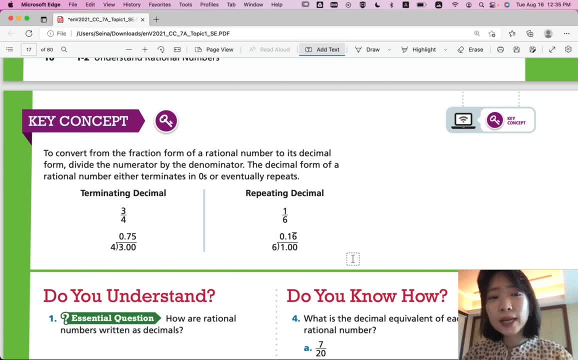 it's not a rational number. okay, guys, that was lesson 1-2, understanding rational numbers. well, if you have any more questions, please ask Ms King in class. we'll continue with the next lesson in the next video. thanks, bye.